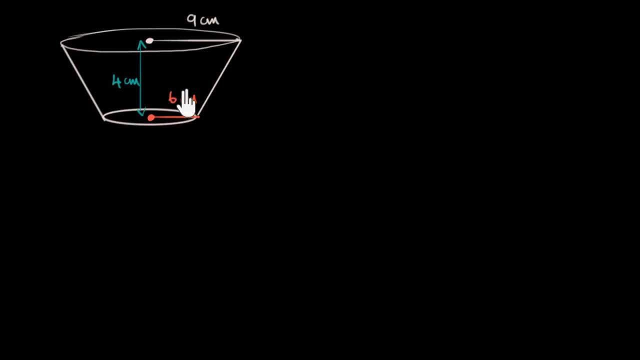 care about this. shape like this is not one of the common shapes, right? this is not a cone, this is not a cylinder, but it's something in between a cone and a cylinder, if you think about it, because it is like converging like this, but not completely all the way to become a cone. 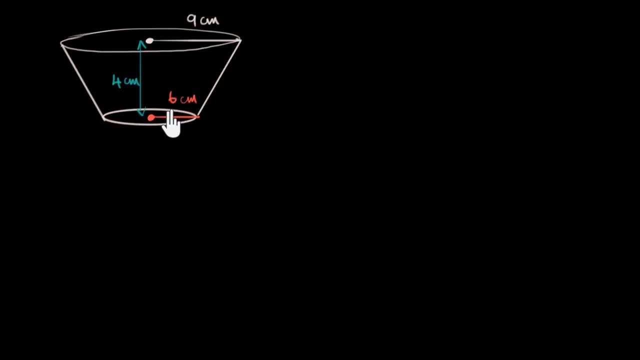 we call this a frustum of a cone. i like to just think of it as a bucket or a, or a tumbler or an ice cream cup, and i think that we uh, specifically study this shape because this is pretty common, right? a bucket is a common shape, and the amount of water a bucket holds is something that you. 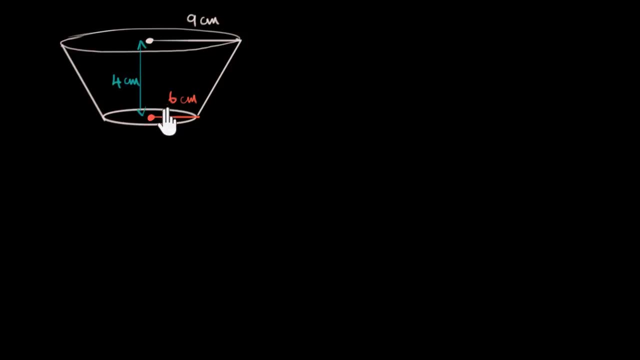 can actually care about in the real world. so how do you do this? um, you can go ahead and maybe, like, look up the formula. somebody has derived it for this particular shape. it's called the itself. if you put in this length, this length and this length. but if you're like me, if you, 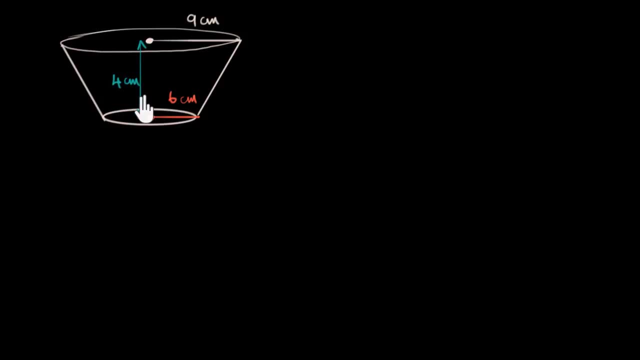 don't remember it, or if you don't know it, or if you don't like to remember it. the way to do this is to do what we're doing for all the other problems, which is, look at this shape that's a little unfamiliar and ask: can i represent it as solids that are familiar to me and in 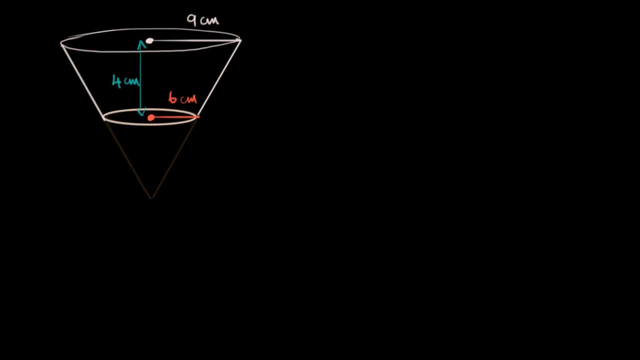 this case, the answer is yes. you can just imagine it to be made of a bigger cone from which a smaller cone has been cut out, so a large shape that's familiar for a bigger cone from which a smaller cone has been cut out. so a large shape that's familiar. for what? 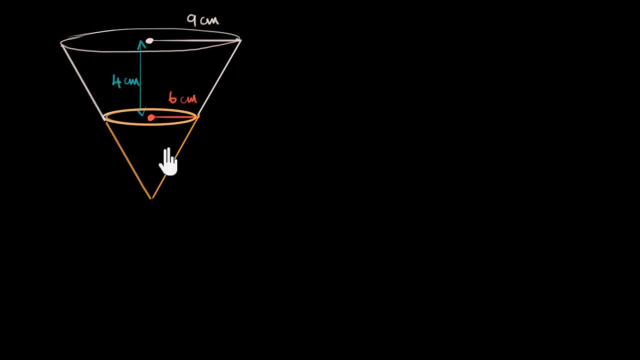 which we know the formula. we spend some time remembering the formula for the volume of a cone right. it's 1 by 3 pi r squared h, so we remember that. so find the volume of this larger cone, subtract the volume of the smaller cone and you'll get the volume of this. now, that's the strategy you. 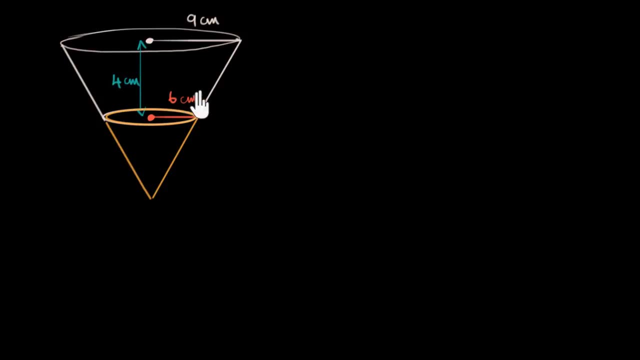 can go ahead and do it, except that there are some lengths missing, right, if you notice. i'm just gonna label this now, if you notice, to do that, i need the height of the smaller cone and i need the height of this bigger cone, both of which have not been given to me directly now. i say directly because they 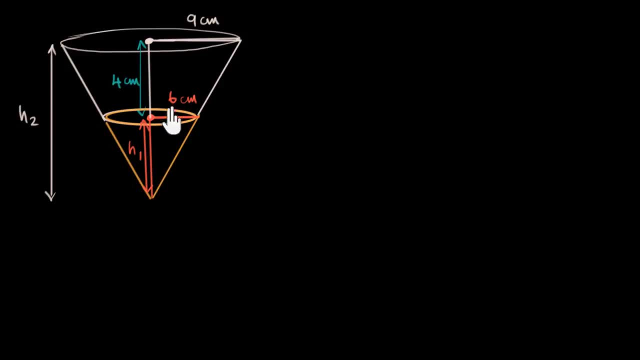 have been given to me indirectly, like the moment i see this length, this length and this, this height given to me. there is only one bucket i can have with these dimensions, which means there is only one cone i can draw. that completes them. but how do i find this height? h1. 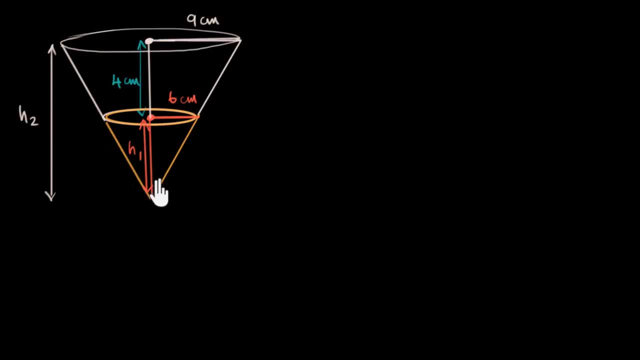 the observation i make is this triangle over here. i know this is a cone, but if you look at it right, right from front, in other words, you look at a cross section- this will be a triangle, this will be a triangle and they will be similar triangles. this angle is equal and this is 90. this is 90, so 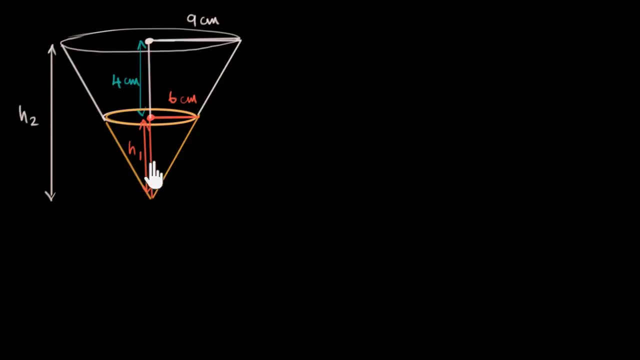 a, a similarity. if you want to be precise about it, then what we can do is write: this side by this side will be equal to this side by this side. the reason this should strike me is that i'm looking for a relationship such that which i can use some equation that i can form that will connect my 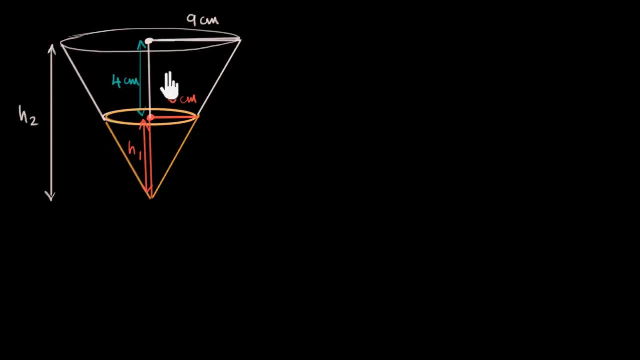 unknowns, one to my knowns over here. so now i can actually go ahead and write that equation. what would it be? h1 by 6, or i can. or i can write it the other way as well. i can write: h1 by h2 will be 6 by 9, that's. 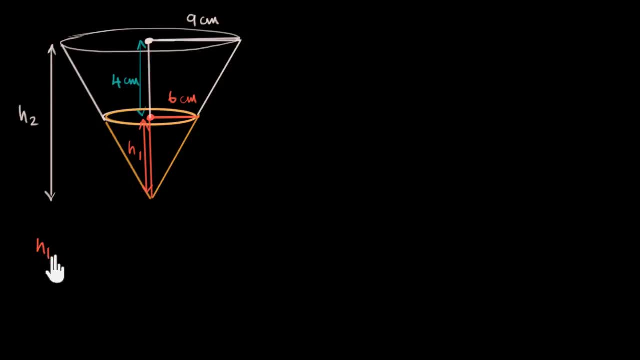 another way of another way of writing it. so i'm going to write that h1 by h2 equals. so my unknowns on one side and i have my knowns on the other side- 6 by 9. now a good thing is h2 is not independent of h1, right, it's just h1 plus 4, so i can go ahead and 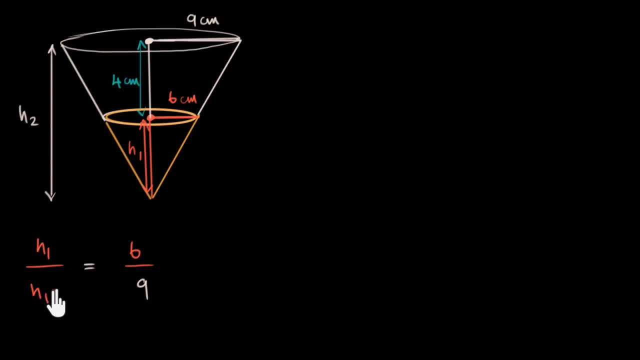 write h2 as h1 plus 4, which means i will reach that state that i like, which is one equation, one unknown. i know that's solvable, so i can just cross, multiply and find the answer. so it's going to be: 9 h1 equals 6, h1 plus 4 into 6, so 6 h1. 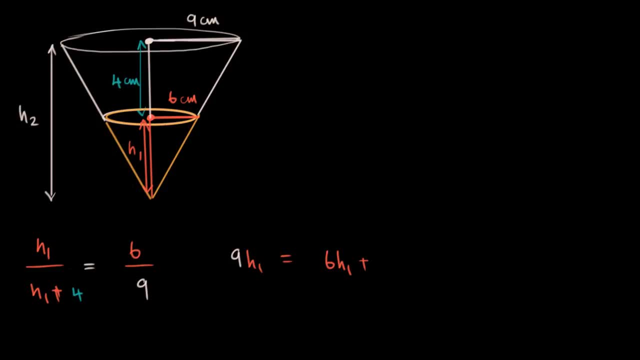 so plus 6 into 4, that is 24. now i can subtract 6 h1 on both sides. that will give me 3 h1 on this side and 24 on this side, which finally gives me h1 equals 8 centimeters. notice that this is the key idea. the key idea is being able to visualize this cone over here. 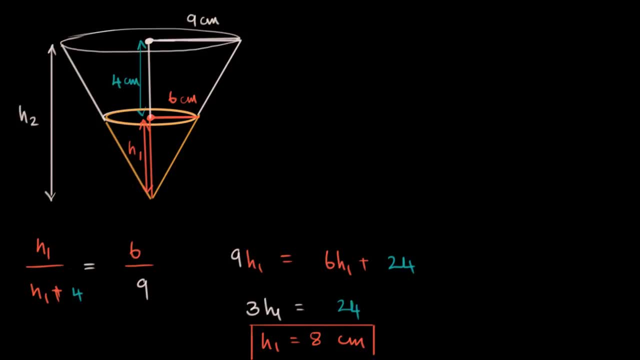 using similarity to find h1 plus 6 into 4, that is 24. now i can subtract 6 h1 on both sides. that will give me 3 h1 on this h1 over here, with which you can find h2. h2 equals: this is 8, this is 4. so this is 8 plus 4, or? 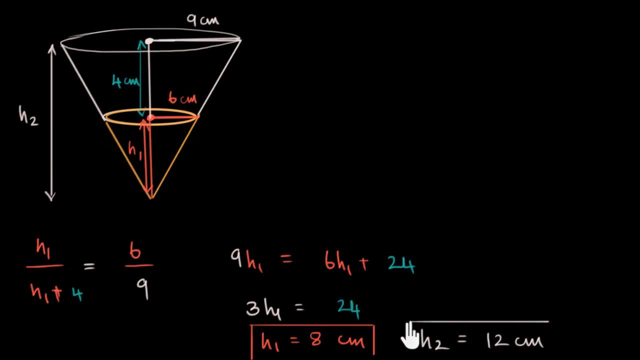 12 centimeters and you have done all of the hard work. you need to solve this problem, because now it's just about writing the volume of this bigger cone, which is 1 by 3, by r2 squared. i'm going to call this large radius r2, r2 squared, h2. 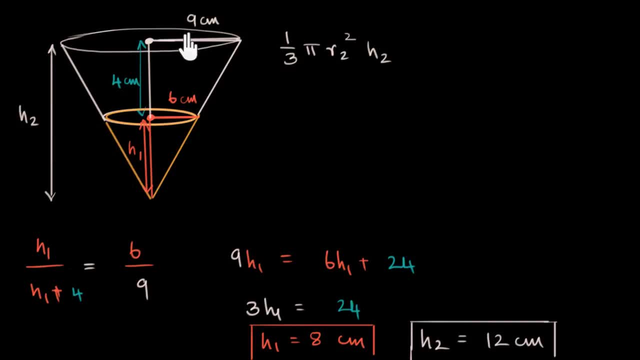 that is the volume of this big cone. i want to subtract from this the volume of the smaller cone, which is 1 by 3 pi r1 squared. i'm going to call this small radius r1 squared, h1. now notice that you have all of this: r2 is available, h2 you found, r1 is available and h1 you found, which means now. 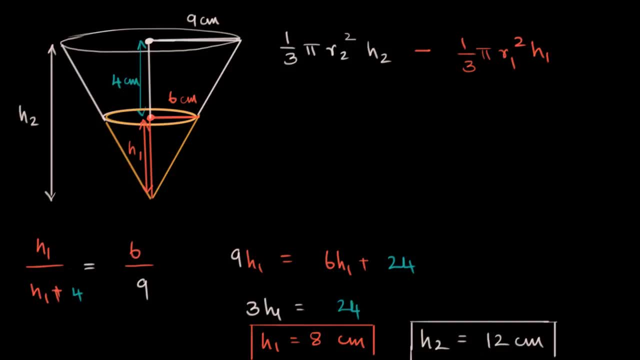 this boils down to doing the calculation without making any mistake. now, let's do that. so 1 by 3 into pi can be taken out common sense. now, let's do that. so 1 by 3 into pi can be taken out common sense. 1 by 3 into pi, i'll take it as 22 over 7. let's maybe draw a line here so that we know that this. 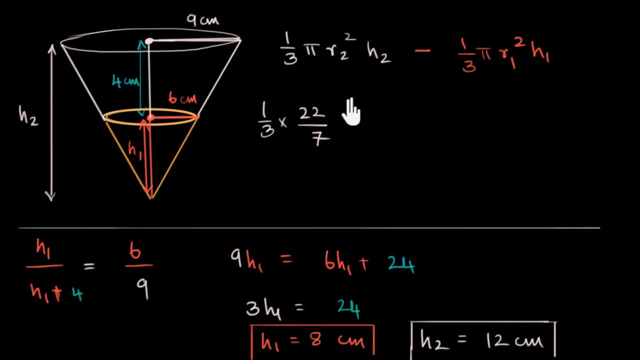 is where we did that calculation. this is where we are finding the volume and this can be multiplied by r2 squared, which is 9 squared. 9 squared multiplied by. i'm going to write 81 for 9 squared, 81 into h2, which is 12. 81 into 12, that looks like 81.12 minus. 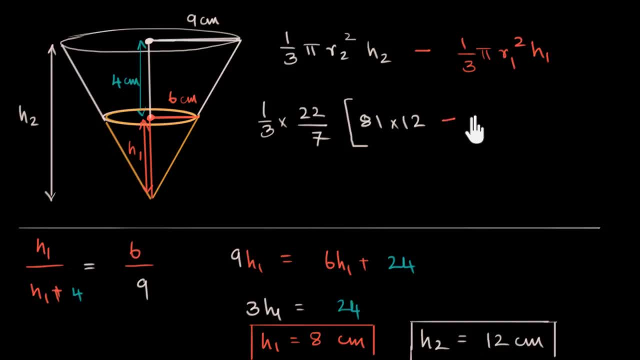 uh, r1 squared, which is 6, squared, that's 36, 36 into h1, which is 8 centimeters into 8. now you can notice everything. here is a number. whatever you get in centimeters, cube will be the answer. now you can go ahead and do this calculation. maybe you can take something out. 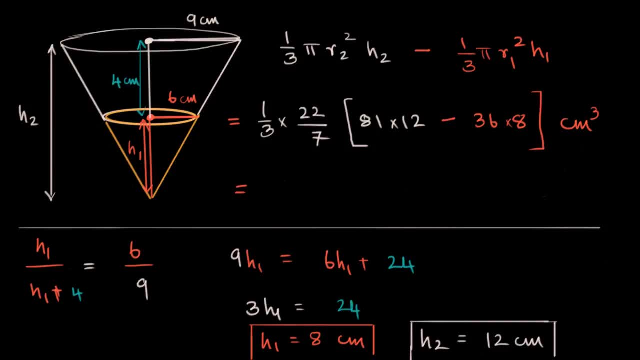